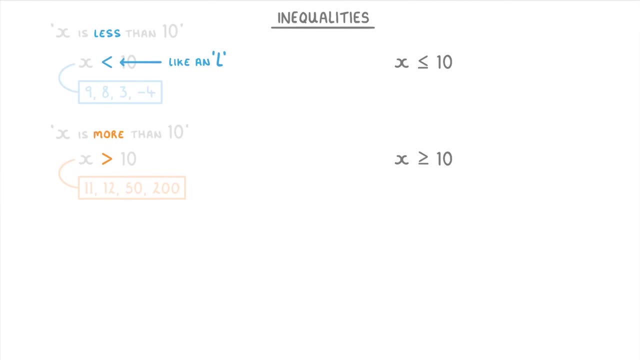 The next thing we need to look at are these two symbols, which look pretty much the same as our less than and more than signs, except they also have these horizontal lines underneath them. The straight lines basically mean or equal to. So this first expression means that x is less than. 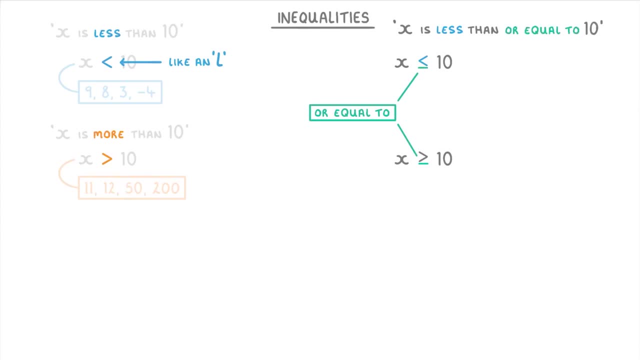 or equal to 10.. So, as well as being numbers like 9,, 8,, 3, or negative 4,, x could also be 10 itself. Similarly, the second expression means that x is more than or equal to 10.. So again, 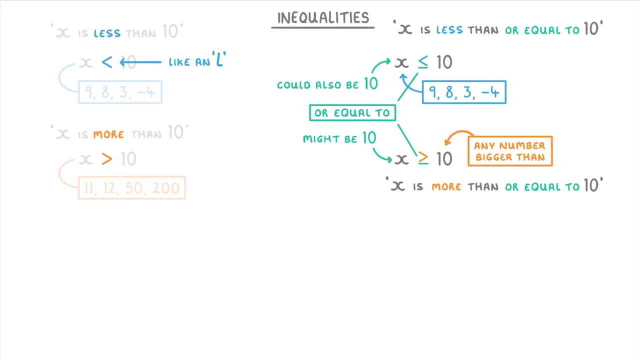 the number might be 10 itself, or any number bigger than 10.. Another important thing to know is that when we take an expression like x is less than 10,, that means exactly the same thing as 10 is more than x, And in both cases we're saying: 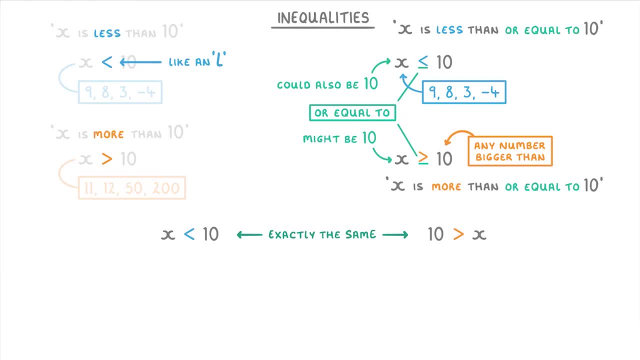 that 10 is the bigger value and x is a smaller value. We can also use negative numbers with inequalities. For example, x is a small number, so we can'tій is less than negative. 5 means that x can be any value smaller than negative 5.. For example, 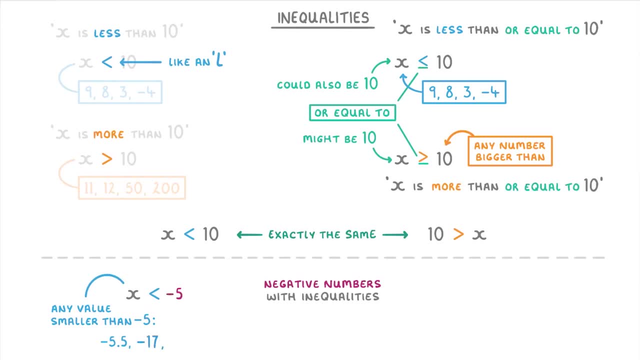 negative 5.5,, negative 17,, negative 100, and so on. Whereas if x was bigger than or equal to negative 5,, then it could be negative 5 itself, or anything bigger like negative 2,, positive 2, or positive 50.. 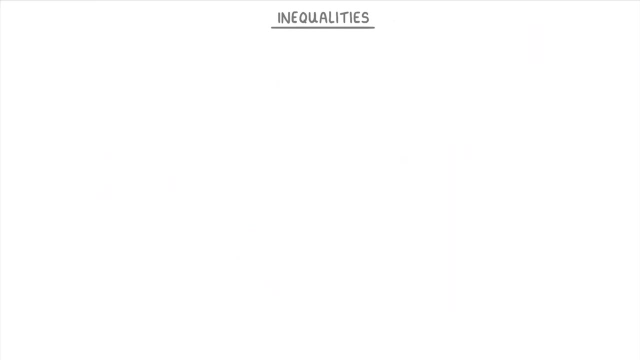 The last thing we need to cover are inequalities like this, which contain more than one inequality sign. The signs work in exactly the same way, though, So this one just means that 3 is less than x and that x is less than or equal to 7.. Or in other words, x has to be between 3 and 7.. 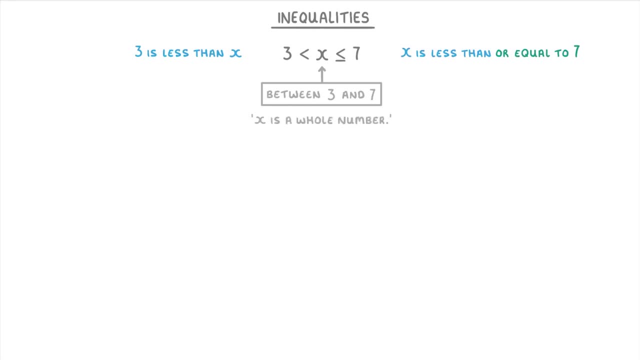 So if we were told that x is a whole number, then x must be 4,, 5,, 6, or 7. Because, remember, it can't be 3 itself, because 3 is less than x, but it can be 7 itself. 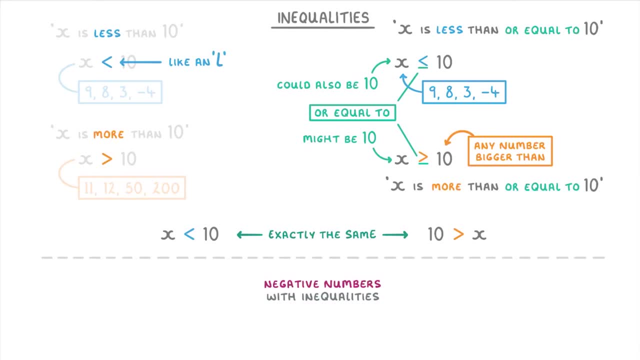 We can also use negative numbers with inequalities. For example, x is less than negative 5,, which means that x can be any value smaller than negative 5.. For example, negative 5.5,, negative 17,, negative 100, and so on. 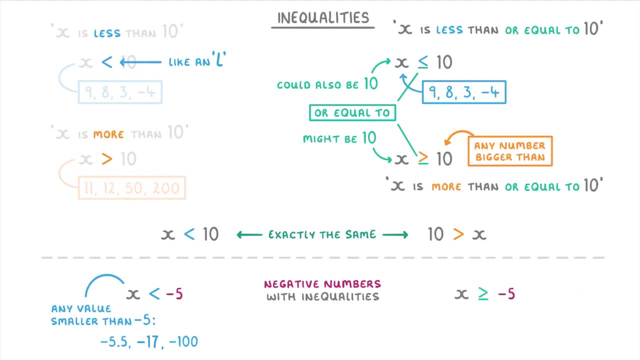 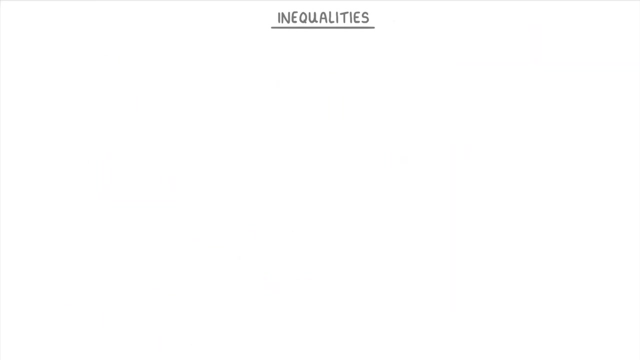 Whereas if x was bigger than or equal to negative 5, then it could be negative 5 itself or anything bigger like negative 2,, positive 2, or positive 50.. The last thing we need to cover are inequalities like this. 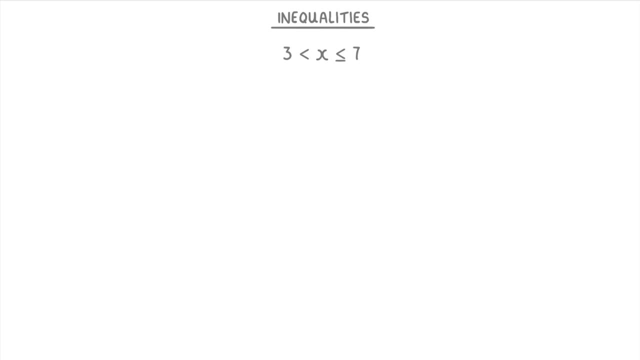 which contain more than one inequality sign. The signs work in exactly the same way, though, So this one just means that 3 is less than x and that x is less than or equal to 7. Or, in other words, x has to be between 3 and 7.. 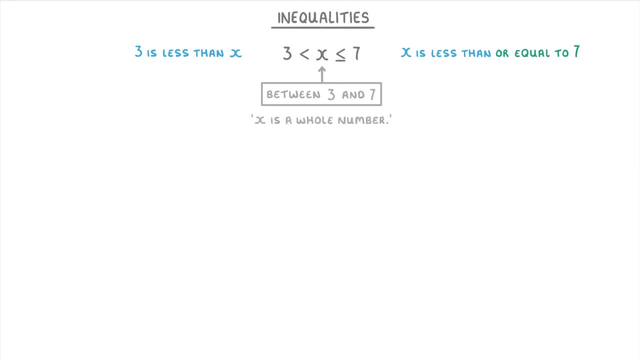 So if we were told that x is a whole number, then x must be 4,, 5,, 6, or 7. Because, remember, it can't be 3 itself, because 3 is less than x, but it can be 7 itself. 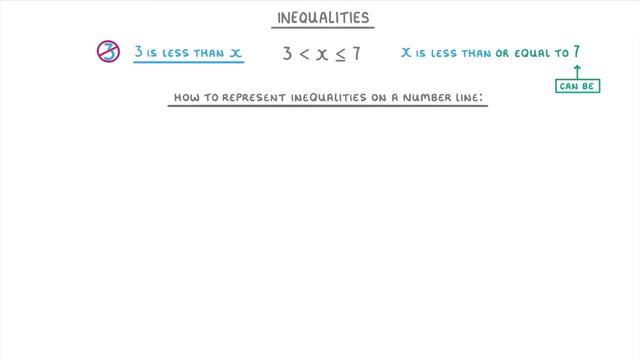 You also need to understand how to represent these inequalities on number lines. So for this one, if we look at this number line of 0 to 10, x must be somewhere in this region between 3 and 7.. So we put little circles above the 3 and the 7.. 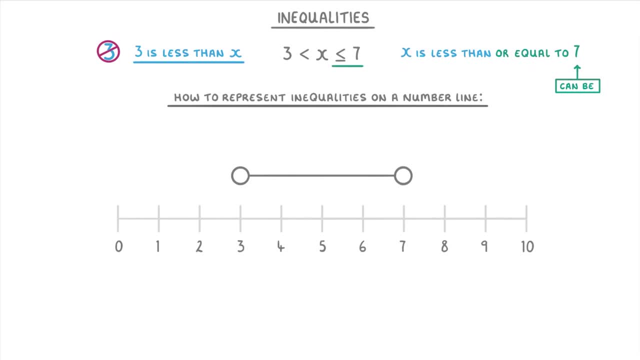 The important bit, though, is that, because x can also be equal to 7 itself, we need to colour in this circle on the right, which tells us that x can be 7.. Whereas, because x can't be 3,, we leave the circle above 3 empty. 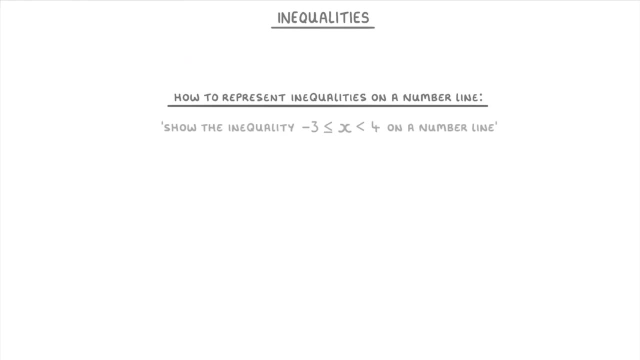 Let's have a go at one more. So for this question we need to show the inequality: negative 3 is less than or equal to x, which is less than 4 on a number line. So if we draw a number line from minus 5 to positive 5,, 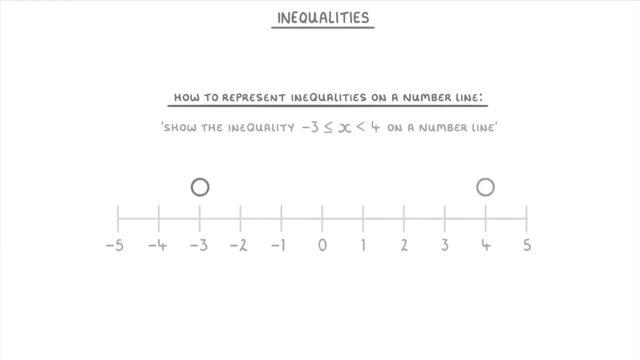 then we can put little circles above the minus 3 and the 4, and join them up with a line. Then the last thing we need to do is check if we need to fill in either of our circles. So, because it says that negative 3 is less than or equal to x.